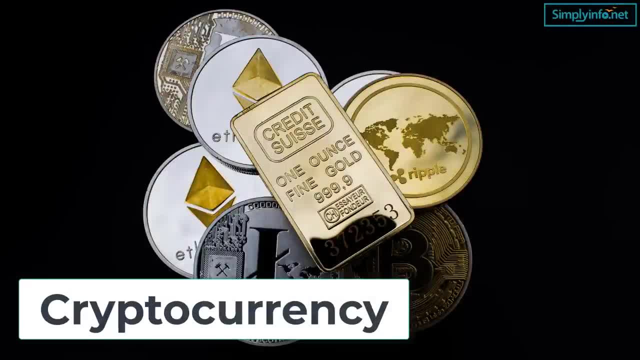 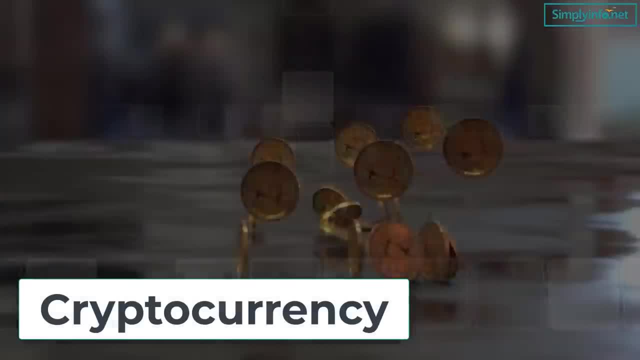 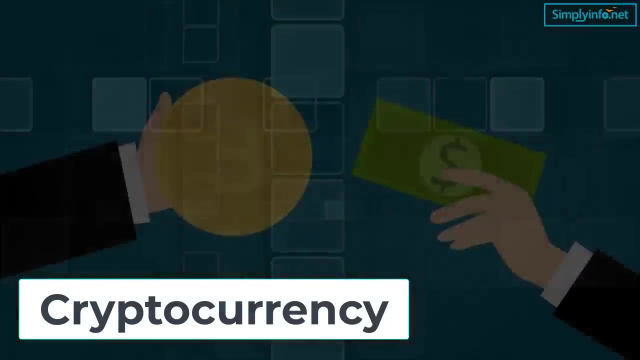 Cryptocurrency is the digital currency that has the true worth. Cryptocurrency is a form of payment that can be exchanged online for goods and services. Many companies have issued their own currencies, which are often called as tokens, and these can be traded specifically for the goods and services provided by that company. 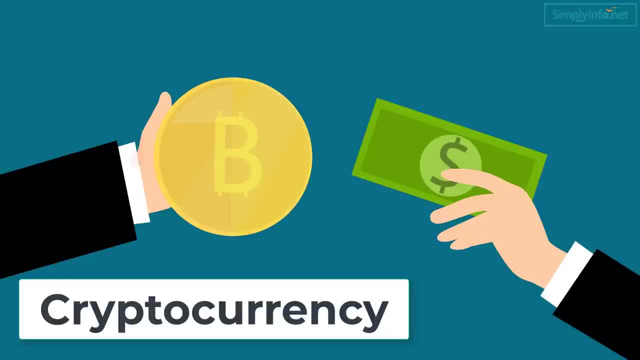 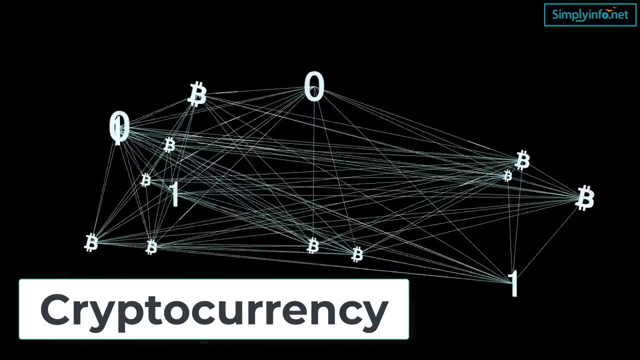 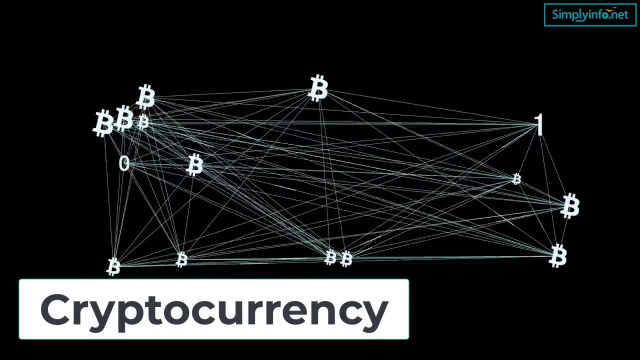 One needs to exchange Real currency for the cryptocurrency to access the good or service. Cryptocurrency work using a technology called blockchain. Blockchain is a decentralized technology which is spread across many computers that manages and record transactions. Blockchain is a specific type of database. 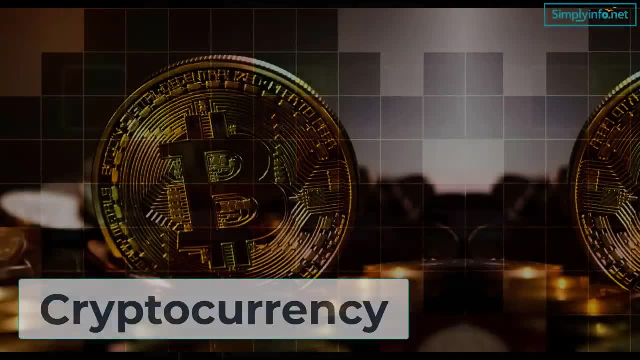 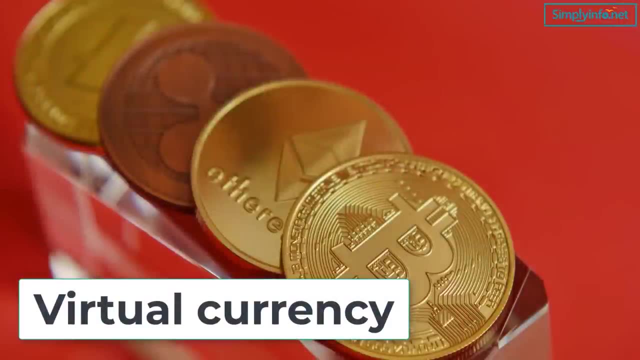 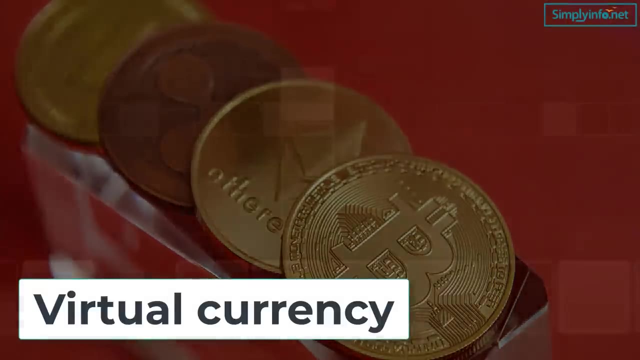 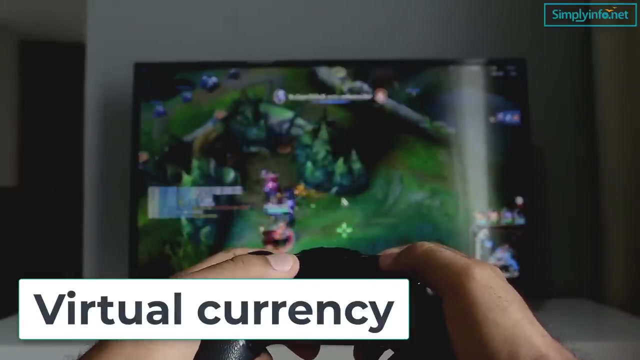 It stores data in blocks that are then chained together. Virtual currency. Virtual currency is a type of unregulated digital currency. It is a digital currency that is utilized inside a particular network. It is not issued or controlled by a central bank. For example, all FarmVillay players approach in-game virtual money coins with which they can buy things for their ranch. 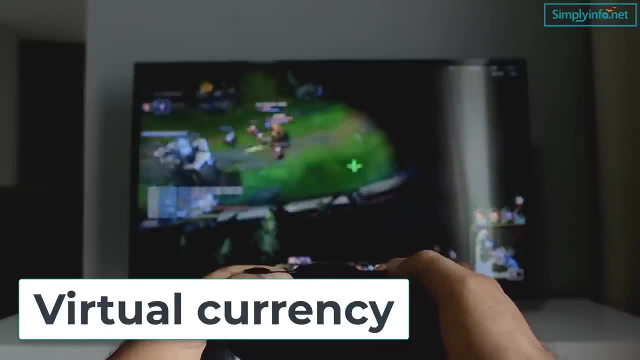 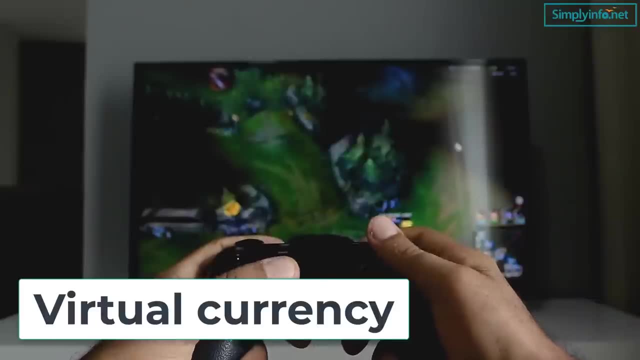 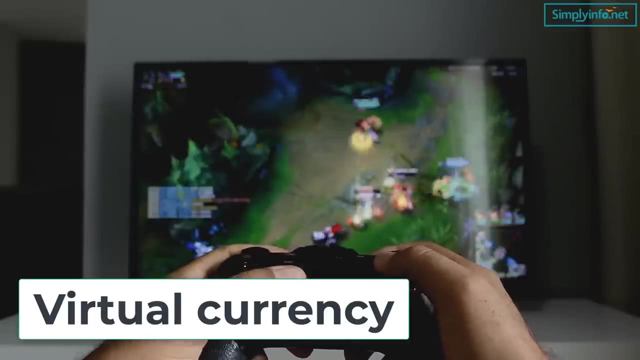 Virtual currencies are typically issued by private issuers and used amongst specific virtual commodities. It is just substantial. inside the predefined network, One cannot take the FarmVillay coin. It can be used to buy something from McDonald's. As a result of its unregulated nature, a virtual currency can experience extensive price fluctuations. 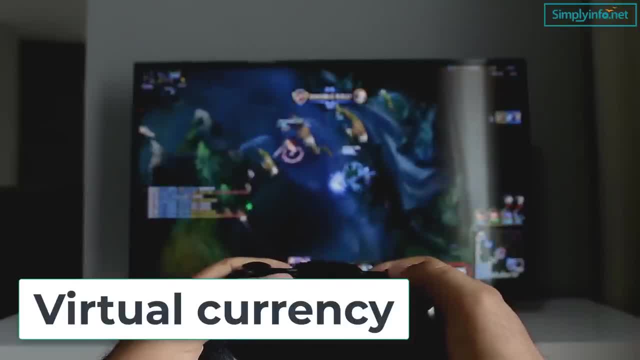 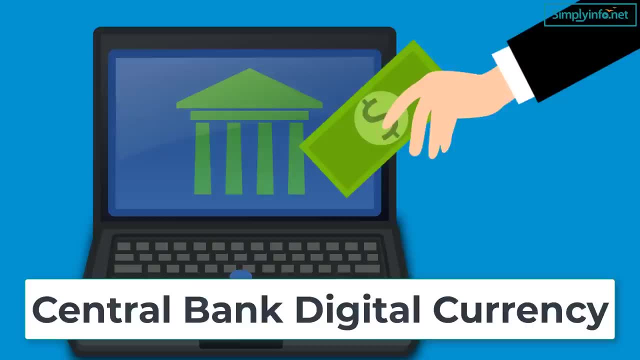 The value of virtual currency is mainly driven by the sentiment of the traders. Central bank digital currency- A central bank digital currency- utilizes technology to represent a country's official currency in digital form. It is also electronic. It is an electronic form of central bank money that citizens can use to make digital payments and store value. 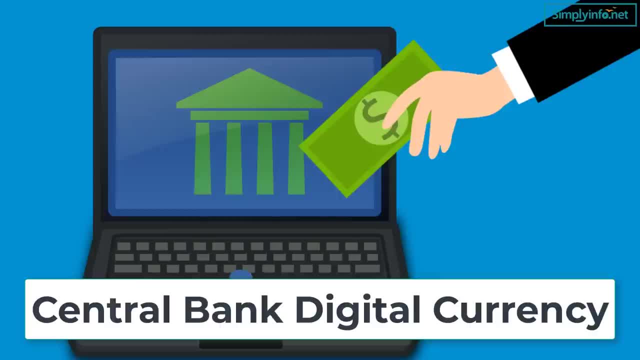 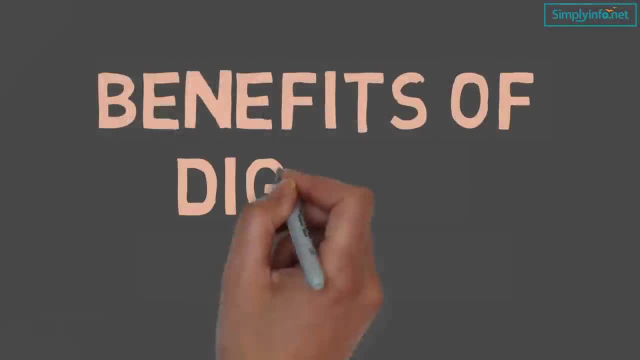 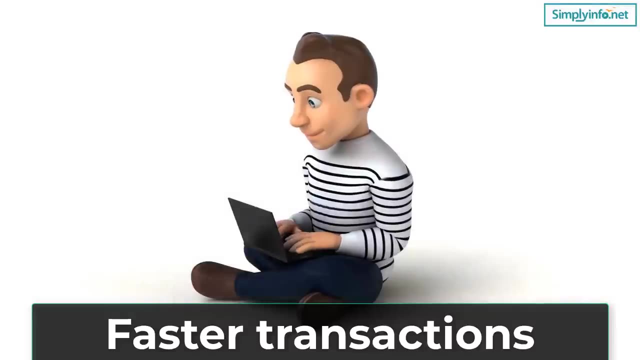 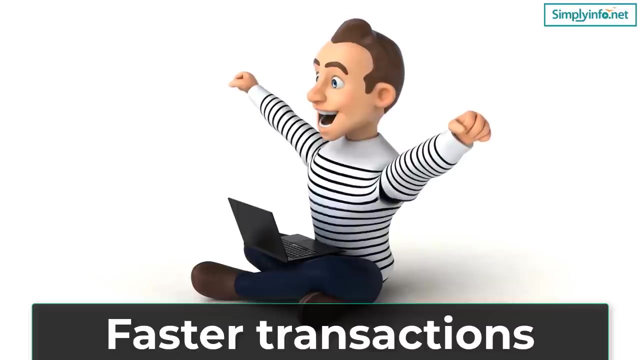 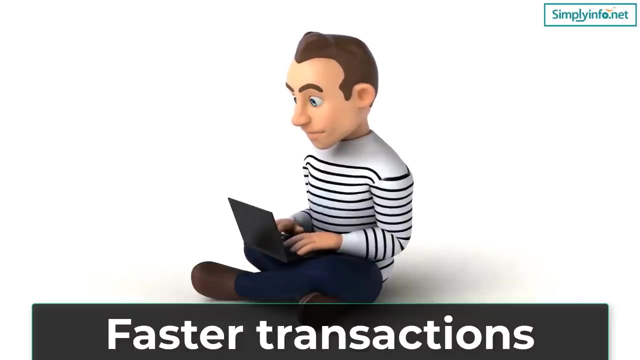 The three main elements of CBDC are: it is a digital currency issued by central bank and it is universally accessible. Benefits of digital currency: Faster transactions. With digital currency one can make transactions immediately without the need for a middleman. For example, if you buy a house, there are many steps that one must go through before the transaction is complete, like getting approval from the bank, etc.